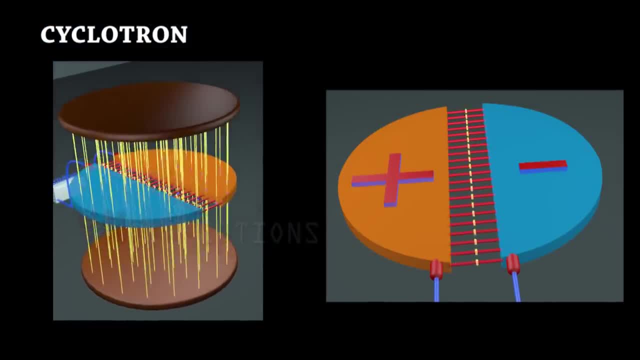 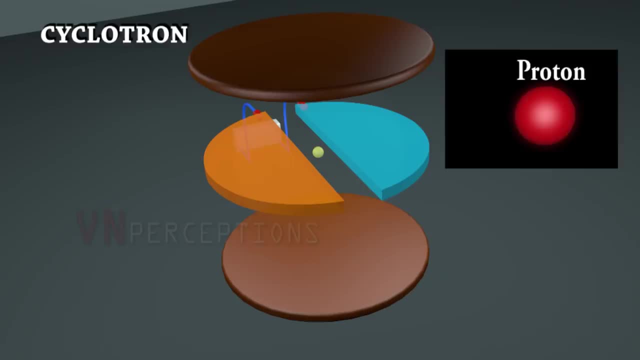 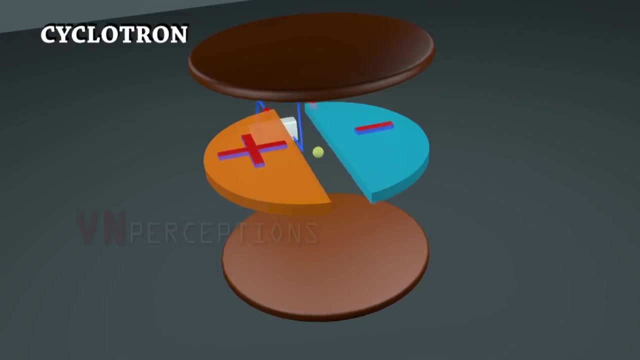 of magnetic field is vertical. When we place a positively charged particle, which may be a proton or a combination of proton and neutron, both since D1 is positive, D2 is negative, there is an electric field between them. Now a force acts upon the charged particle and its direction would be the direction. 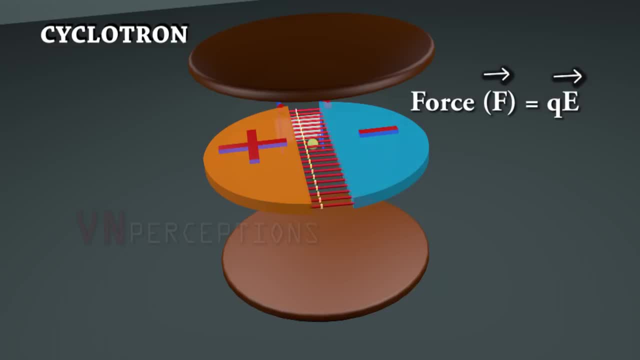 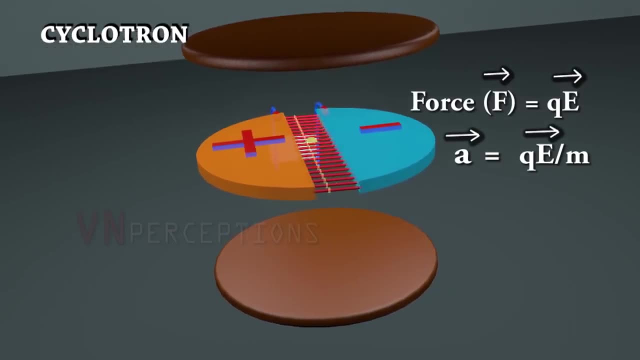 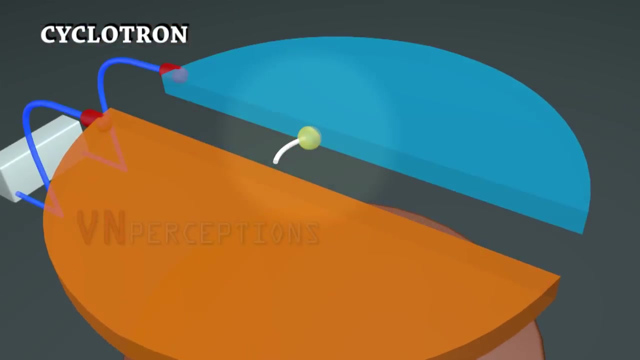 of E. Because of this force the charged particle gets acceleration and because of acceleration the speed increases till it enters the D, Since D is an enclosed container. so the value of electric field is zero. So force becomes zero and acceleration becomes zero. So inside the container there is no electric field. 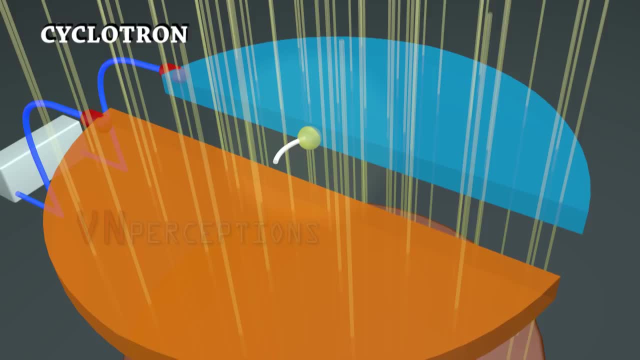 but there is magnetic field and its direction is north. The charged particle now moves perpendicular to the direction of the magnetic field. It experiences a force in a direction perpendicular to the plane containing V and B. This force provides the centripetal force and makes the charged particle move along. 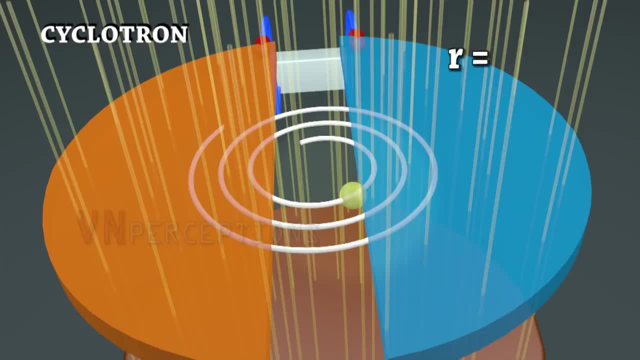 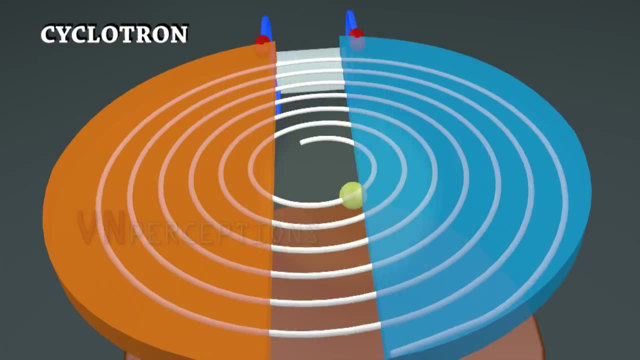 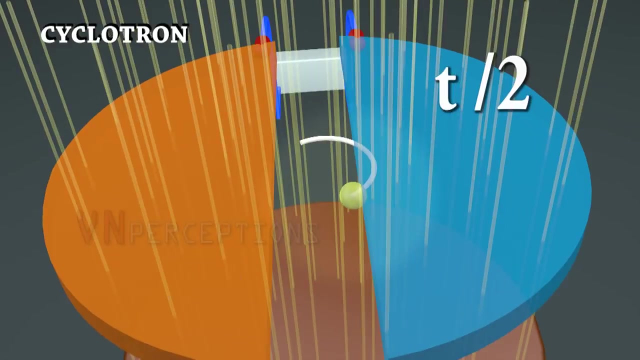 a circular path of radius R is equal to The particle. make a semicircle and comes to the gap, The time taken is t by 2.. Because if the time taken to complete one circle is t, then the time taken to complete semi circle would be t by 2.. 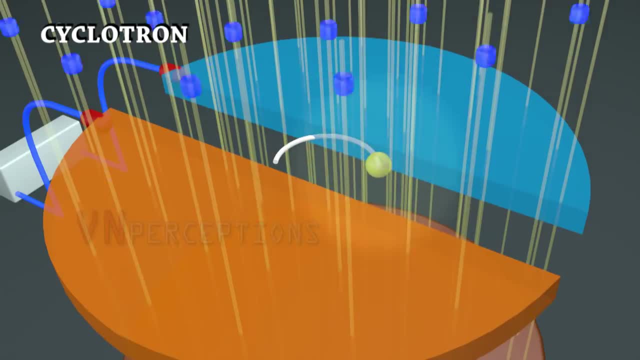 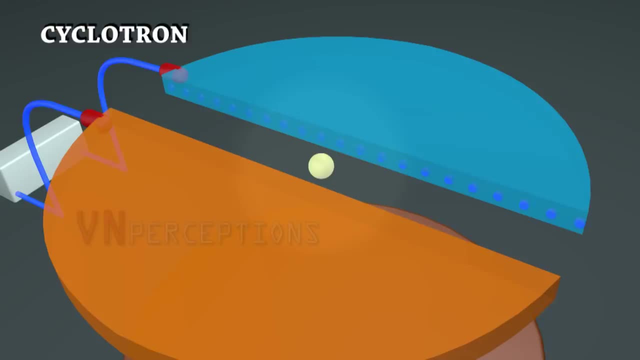 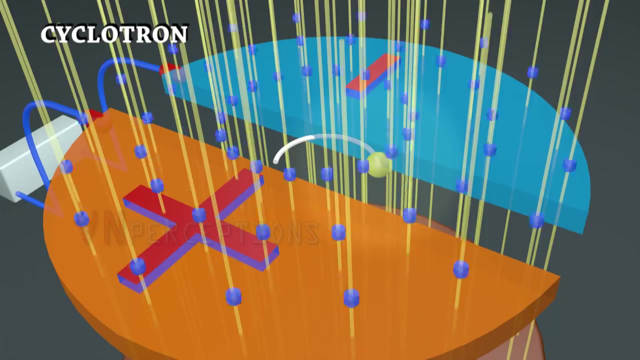 comes to end. it is influenced by electric field. When the particle was born, its velocity was zero. When it enters the D, its velocity is V, and it is constant because the magnetic field cannot change the velocity. The oscillator.